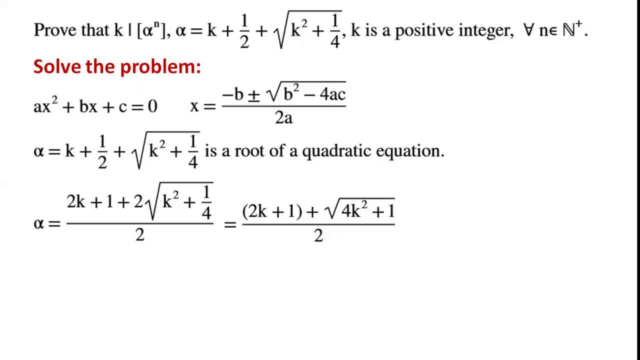 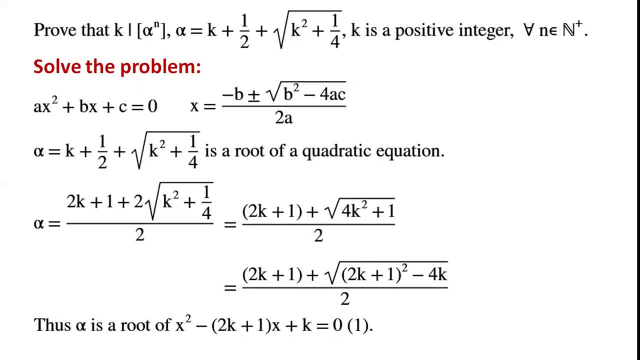 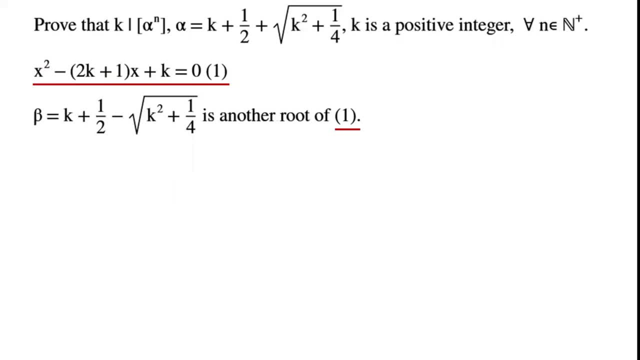 k equals zero. Beta equals k plus a half, minus root of k squared plus a quarter. It's another root of equation one, Since k plus a half, all squared equals k squared plus a quarter plus k. k is the positive integer, So k squared plus a quarter is less than k plus a half. 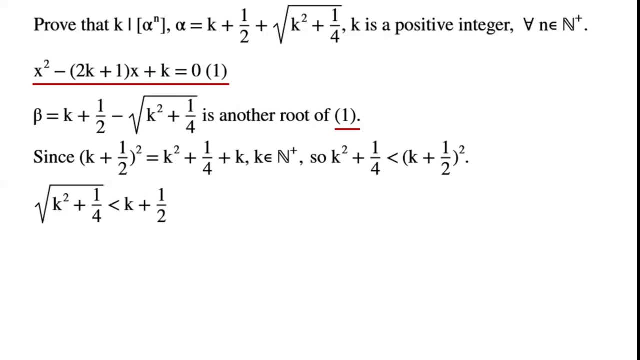 all to the power of two, Which means root of k squared plus a quarter is less than k plus a half. Thus beta is greater than zero. By Vieta's formulas we know that alpha beta equals k. By rearranging the equation, beta equals k over alpha, which is equal to k over k plus. 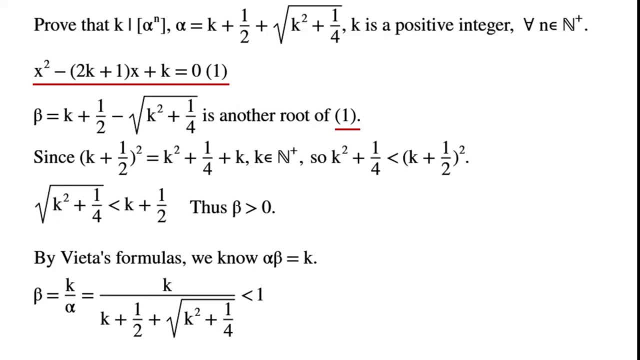 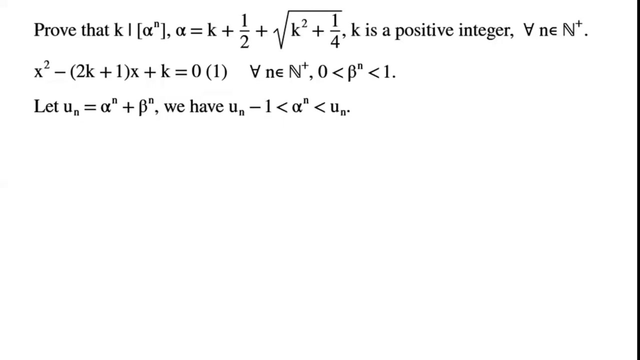 a half plus root of k, squared plus a quarter, which is less than one. Thus, for all n in the set of positive integers, zero is less than beta to the power of n. N is less than one. Let un equal alpha to the power of n plus beta to the. 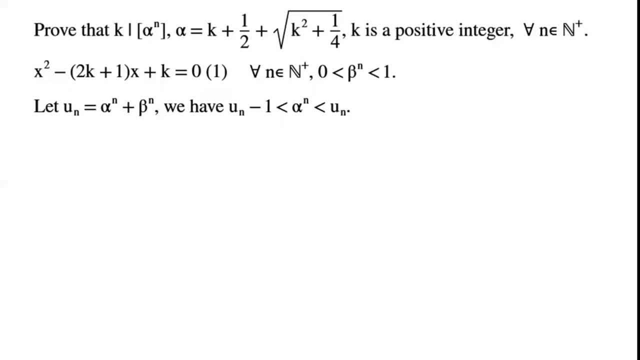 power of n We have. un minus one is less than alpha to the power, n is less than un. If Un is an integer for a and when you convert an power to an integral to n, it's red Alright. so now we have an integer. If we work with a 102 x 90 x 72, zero algebra, it's less than 1.. Let's get all the numbers down and looking at these rhythms in this reading. If one vector per function of an integer is less than one, then a half goes to the power of n, perhaps only 2.. Let's write these numbers very carefully. 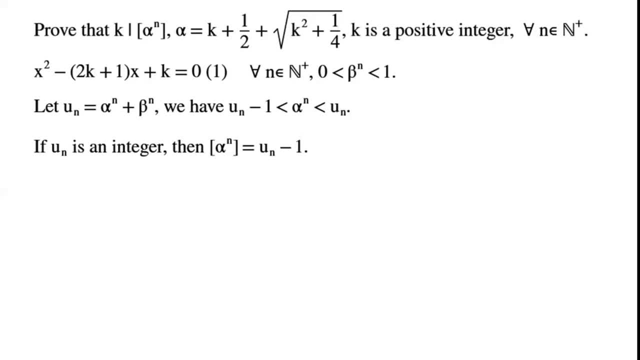 Let's write these numbers very carefully. Then the integral part of alpha to the power of n equals un minus 1.. Thus, proving that the integral part of alpha to the power of n is divisible by k is equivalent to proving that un is an integer and un is congruent to 1 mod k. 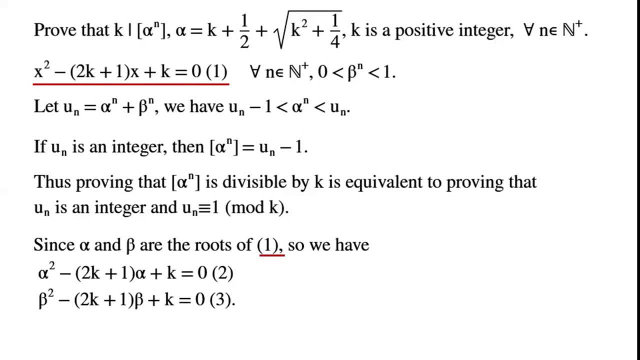 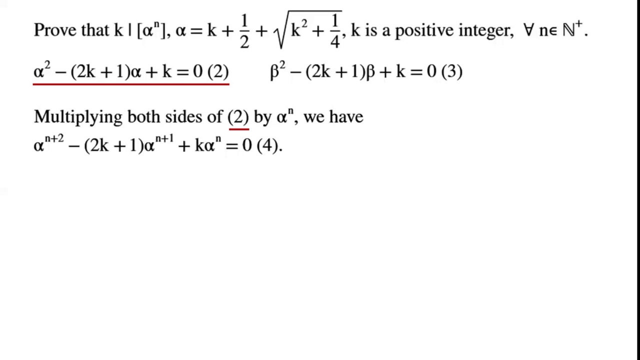 Since alpha and beta are the roots of equation 1, so alpha squared minus 2k plus 1 times alpha plus k equals 0. So beta squared minus 2k plus 1 times beta plus k equals 0.. Multiplying both sides of equation 2 by alpha to the power of n. 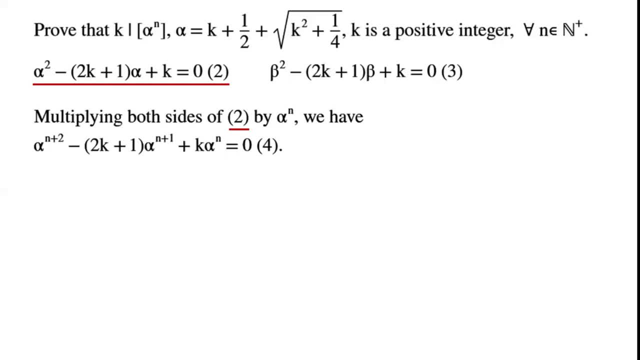 we have alpha to the power of n plus 2 minus 2k plus 1 times alpha to the power of n plus 1 plus k. alpha to the power of n equals 0. Each negative value is the total integral function. So if an integral part of alpha to the power of 3 equals alpha squared minus 1 rule. 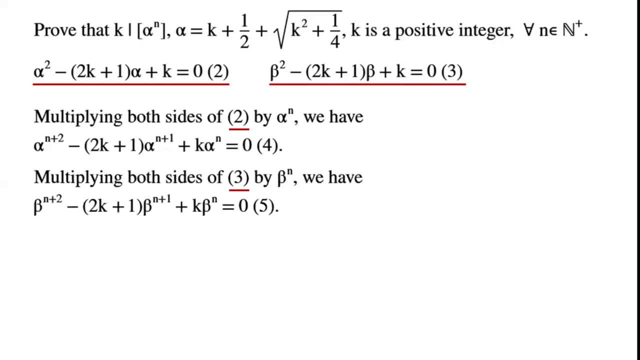 we have the integral part of alpha squared minus 2k plus 1 times alpha to the power of n equals 0.. Because we left out the blockchain rules, we can find them on the hyperlink in the description at the top right side now. 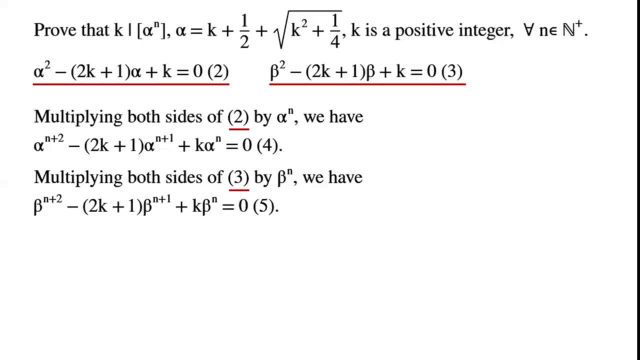 I'm also going to explain how to simplify this into a free copy for the next lesson. But first keep in mind that when we do the correctока وج- quantities, we're not going to write everything in a way to be pulled off. 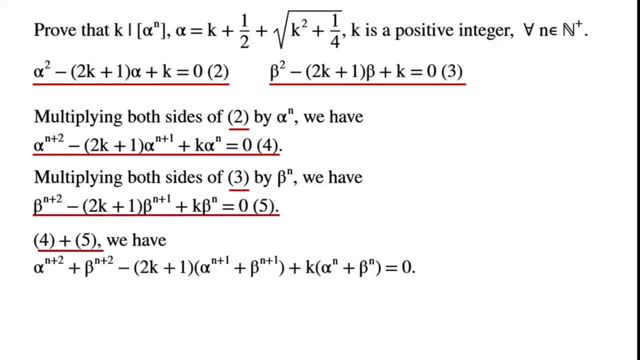 We're going do they in a certain order instead than just 150 of them. Let me do that for another time. Equation 4 plus equation 5. We have alpha to the power of M plus 2 plus beta to the power of M plus 2 minus 2k plus 1 times alpha to the power of M plus 1 plus beta to the power of M plus 1 plus k times alpha to the power of N. 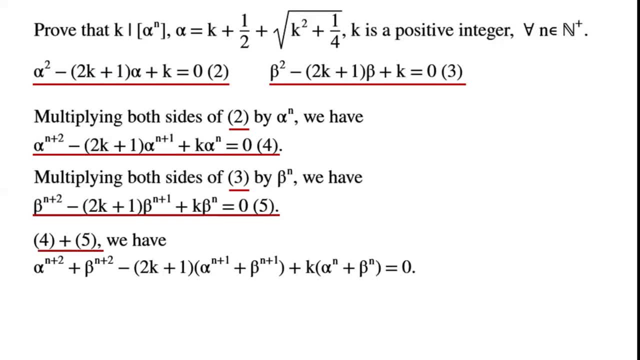 plus beta to the power of n equals zero. alpha to the power of n plus two plus beta to the power of m plus two equals u n plus two. alpha to the power of m plus one plus beta to the power of n plus one equals u n plus one alpha to the power of n. plus beta to the power of n equals u n by. 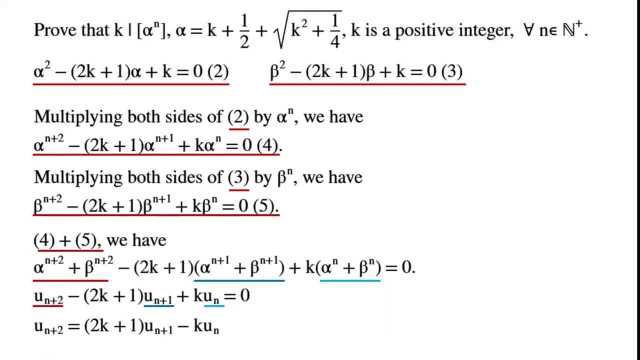 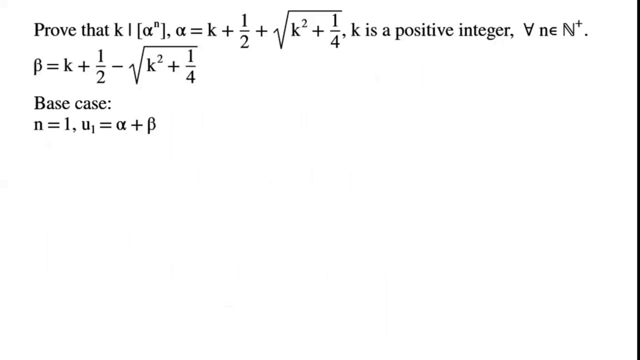 rearranging the equation we have: u? n plus two equals two k plus one. times u? n plus one minus k u n. u n plus two can be written as k times two u n plus one minus u? n plus u n plus one. base case: n equals one u one equals alpha plus beta. 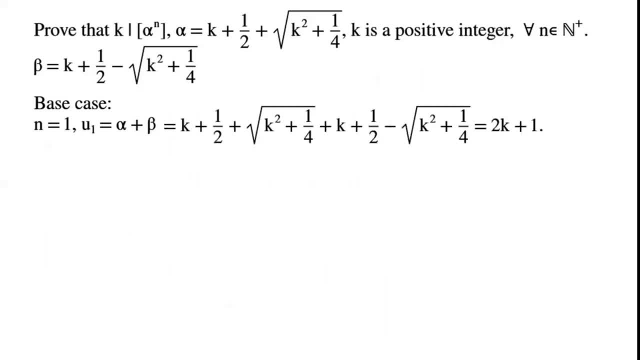 which is equal to k plus a half plus root of k squared plus k times two u n plus one minus u? n plus u n plus one a quarter plus k plus a half minus root of k squared plus a quarter equals two k plus one. thus u one is an integer and u one is congruent to one mod k. 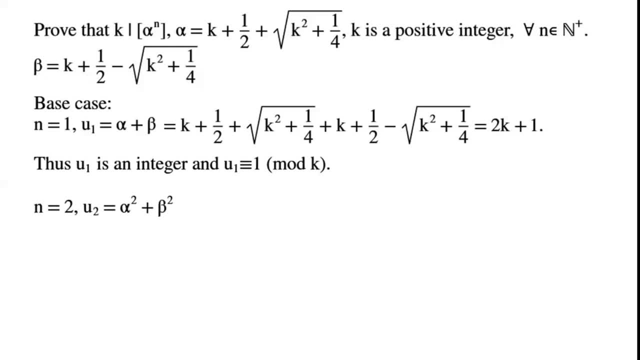 any equals two u two equals alpha squared plus beta squared, equals k plus a half plus root of k squared plus a quarter all squared plus k plus a half minus root of k squared plus a quarter all squared, which is equal to two times k plus a half all. 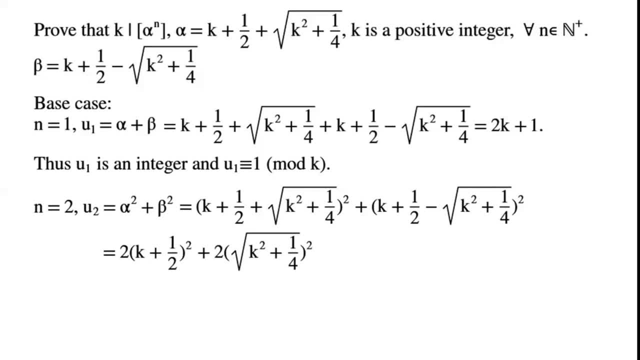 squared plus two times root of k squared plus a quarter, all squared, which is equal to two times k squared plus k plus a quarter, plus two times k squared plus a quarter, which can be simplified to four k squared plus two k plus one. thus u2 is an integer and u2 is congruent to one mod, k. 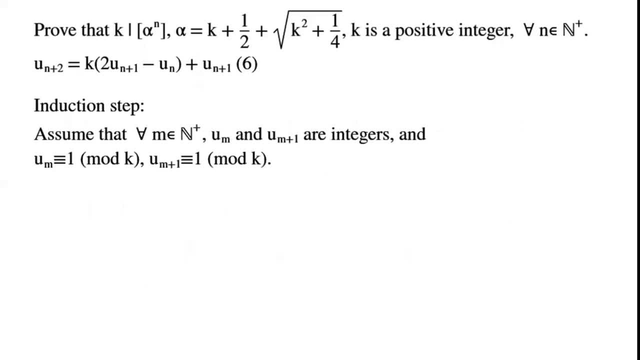 induction step. assume that for all m in the set of positive integers, um and um plus one are integers, and um is congruent to one mod k. um plus one is congruent to one mod k. from equation six we have: um plus two equals k times two um plus one.